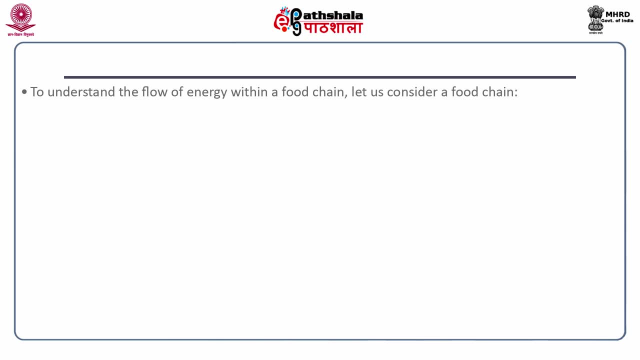 the capability of fixing light energy. To understand the flow of energy within a food chain. let us consider a food chain Here. in this food chain, you will see that this food chain starts with plant. Plants are eaten by the rabbit and rabbit is eaten by the folks. 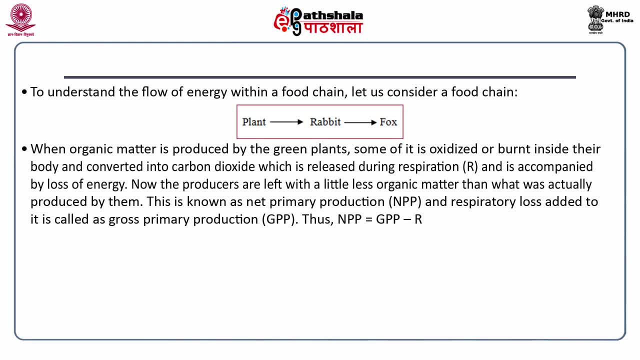 When organic matter is produced by the green plants, some of it is oxidized or burnt inside their body and converted into carbon dioxide, which is released during respiration and is accompanied by loss of energy. Now the producers are left with a 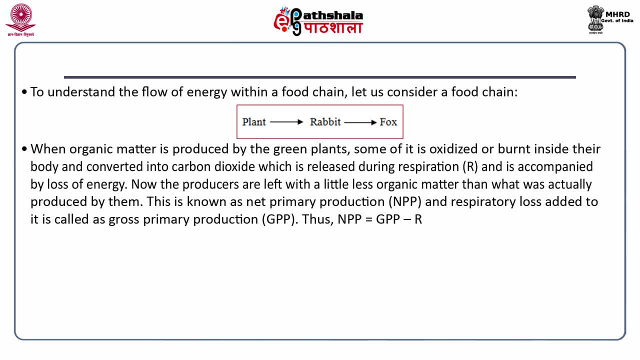 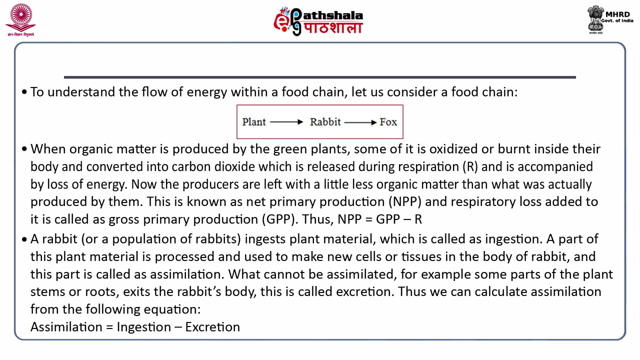 little less organic matter than what was actually produced by them. This is known as net primary productivity, And respiration loss related to it is called as gross primary productivity. So net primary productivity is equal to gross primary productivity minus respiration. A rabbit or a population of rabbits: 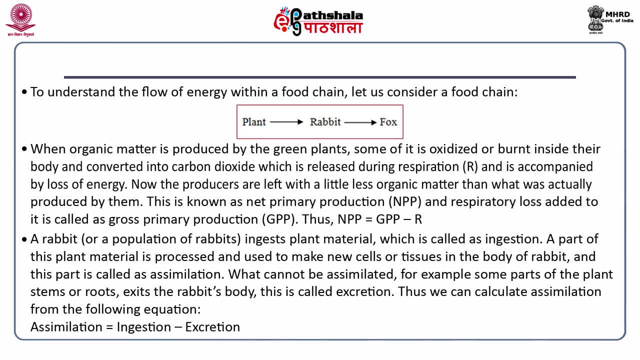 ingest plant material. that is called as ingestion. A part of this plant material is processed and used to make new cells, And this part is called as assimilation. What cannot be assimilated- for example, some parts of the plant, stems or roots exist, the rabbit's body. this is called as excretion. Thus we can. 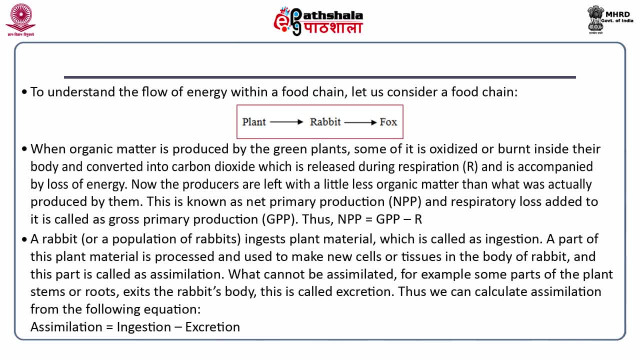 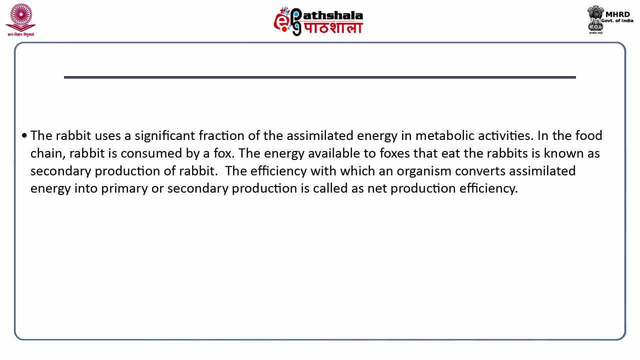 calculate assimilation using the below given equation. that is, assimilation is equal to ingestion minus excretion. The rabbit uses a significant fraction of the assimilated energy in metabolic activities In the food chain. rabbit is consumed by a fox. The energy available to foxes that eat the rabbit is known as: 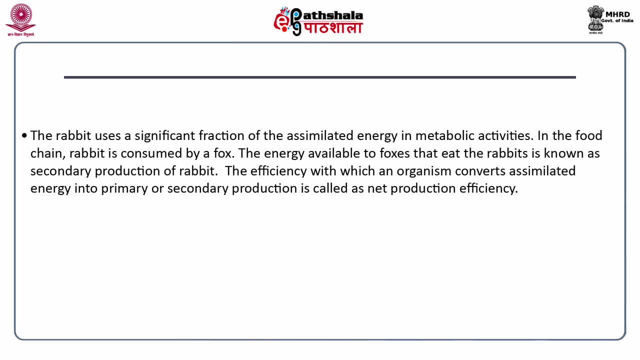 secondary production of rabbit. The efficiency with which an organism converts assimilated energy into primary production or secondary production is called as net production efficiency. This net production efficiency is equal to the production divided by the assimilation for animals, or the net primary productivity divided by the gross primary productivity for plants. The production here refers to growth plus reproduction. 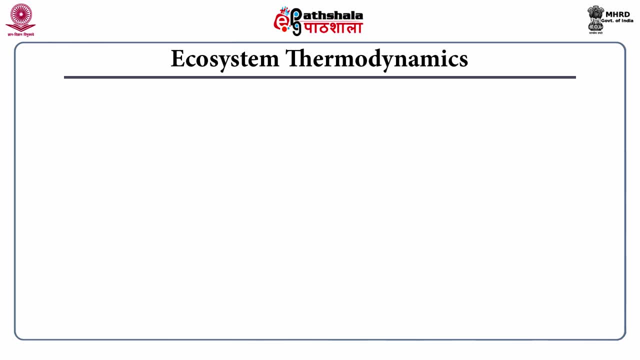 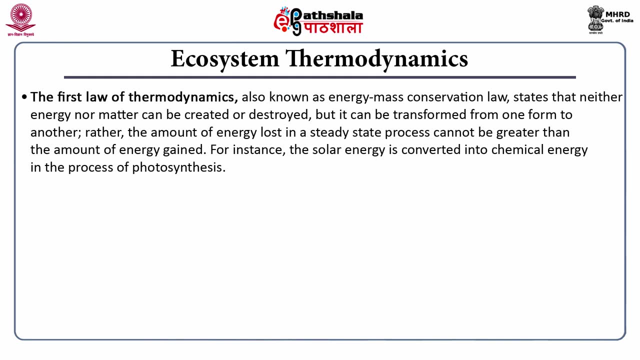 Ecosystem thermodynamics. Let me try to understand little bit about laws of thermodynamics. The first law of thermodynamics, also known as energy mass conservation law, states that neither energy nor matter can be created or destroyed, but it can be transformed from. 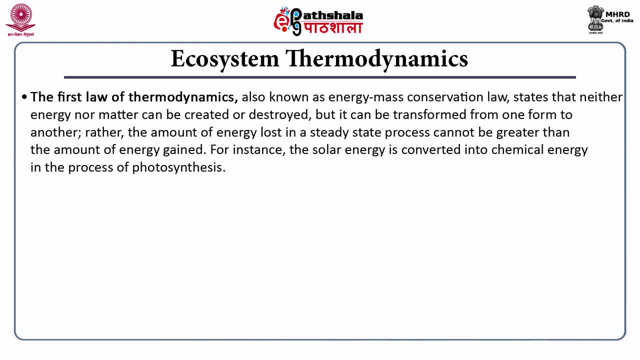 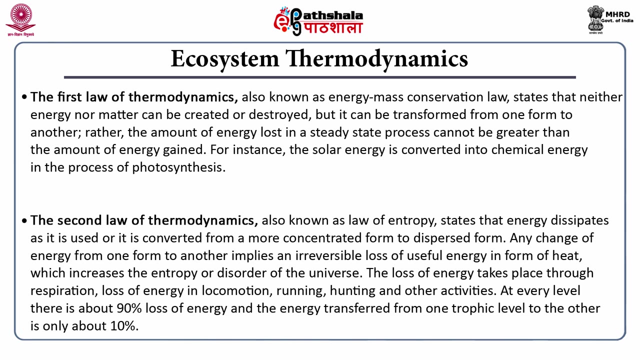 one form to the another form Rather, the amount of energy lost in a steady state process cannot be greater than the amount of energy gained. For instance, the solar energy is converted into chemical energy in the process of photosynthesis. The second law of thermodynamics, also known as law of entropy, states that energy dissipates. 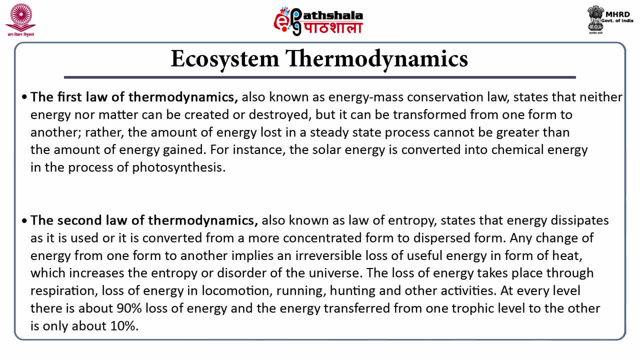 as it is used or it is converted from a more concentrated form to dispersed form. Any change of energy from one form to another implies an irreversible loss of useful energy in form of heat that increases the entropy or disorder of the universe. The loss of energy takes 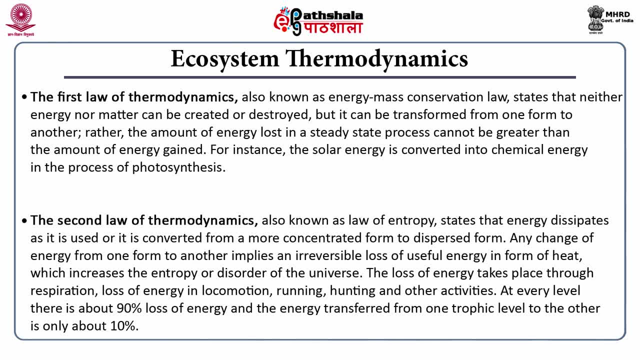 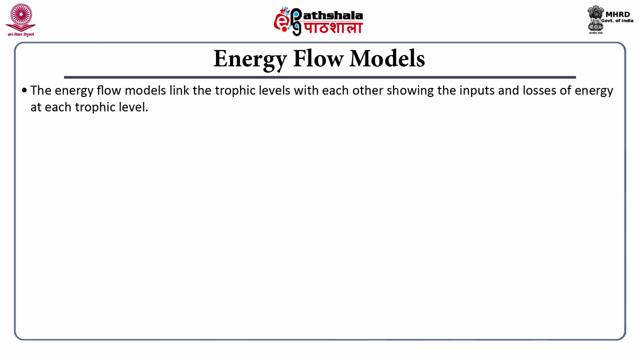 place through respiration, loss of energy in locomotion, running, hunting and other activities. At every level there is about 90 percent loss of energy and the energy transfer from one trophic level to other is only 10 percent. Let we discuss some energy flow models. The energy flow models link the trophic levels. 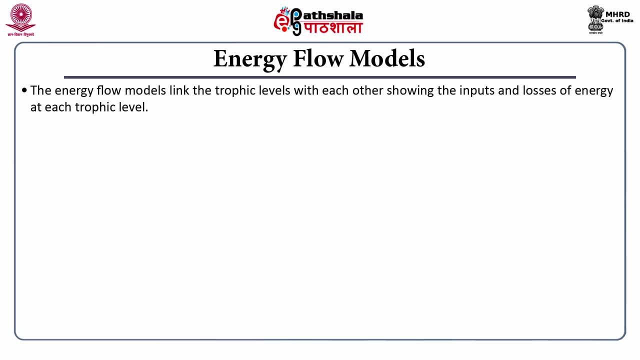 with each other, showing the input and loss of energy at each trophic level. There are several models and we will be discussing them one by one. The first model is a single channel energy flow model. This model is presented on the are shown in this figure. The flow of energy in an ecosystem takes place through the food. 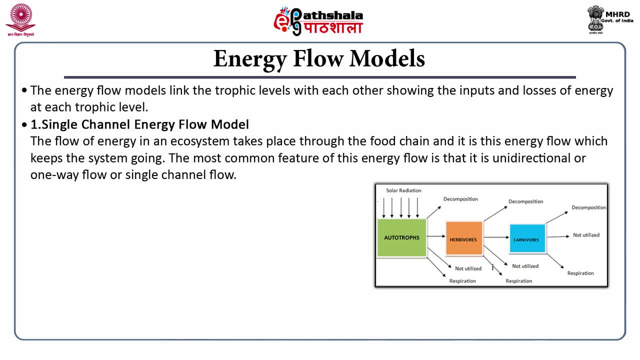 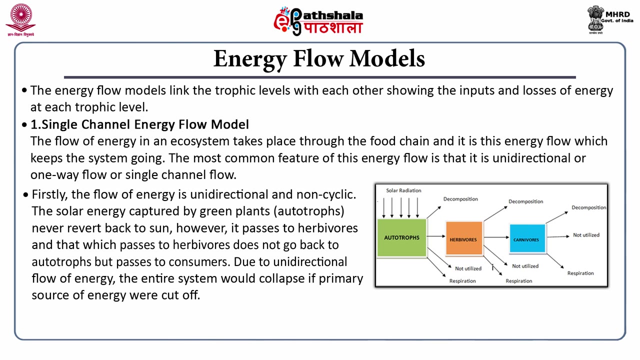 chain, and it is this energy flow that keeps the system going. The most common feature of this energy flow is that it is unidirectional, or one way flow, or single channel flow. Firstly, the flow of energy is unidirectional and non-cyclic. The solar energy captured by 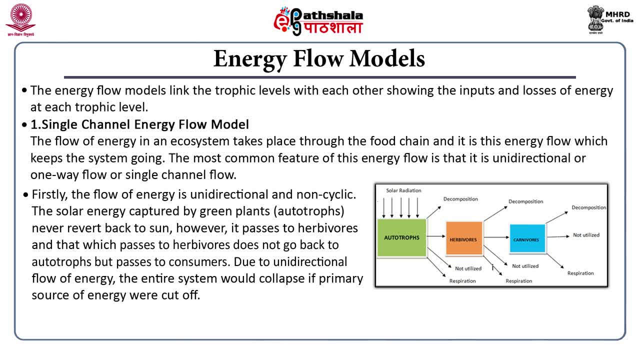 green plants never revert back to sun. However, it passes to herbivores, and that which passes to herbivores does not go back to autotropes but passes to consumer, Due to unidirectional flow of energy. the entire energy flow is unidirectional, So the flow of energy is unidirectional. 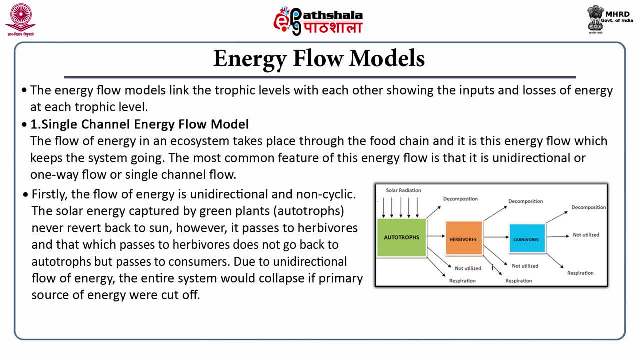 The entire system would collapse if primary source of energy were cut off. Secondly, at each trophic level there is progressive decrease in energy as heat in the metabolic reactions and also some of the energy is utilized at each trophic level. The same is depicted in: 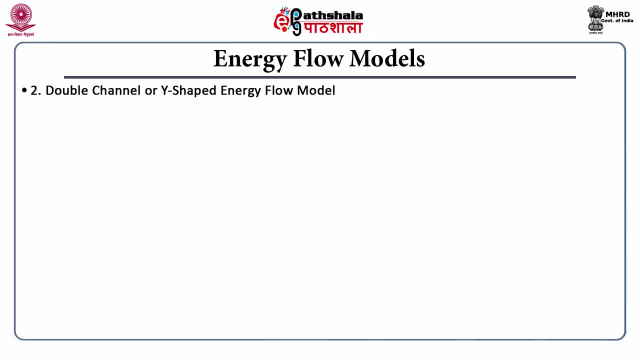 this figure. Second model is double channel or Y-shaped energy flow model. This Y-shaped energy flow model is a double channel or Y-shaped energy flow model. This Y-shaped energy flow model is shown in this figure. The double channel or Y-shaped energy flow model depicts. 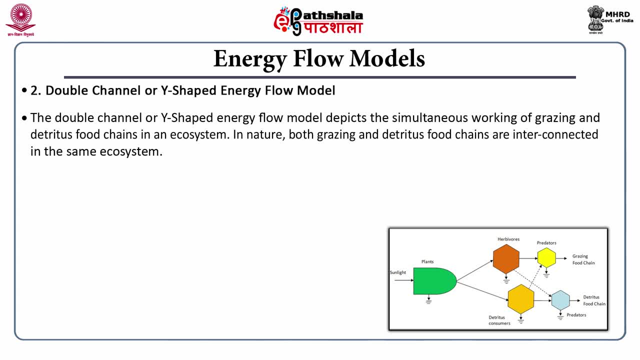 the simultaneous working of grazing and detritus food chains in an ecosystem. In nature, both grazing and detritus food chains are interconnected in the same ecosystem. This we have studied in previous modules. also, Functionally, the distinction between the two is of time lag between the direct consumption of living plants. 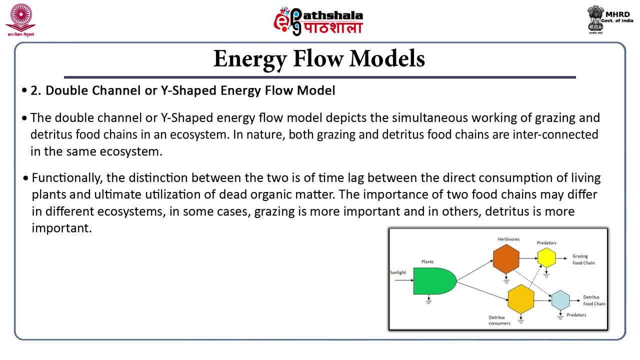 and ultimate utilization of dead organic matter. The importance of two food chains may differ in different ecosystems. In some cases grazing is more important and in others detritus is more important. It happens in marine ecosystems where primary production at open sea is limited and a major portion of it is eaten by herbivore marine animals. 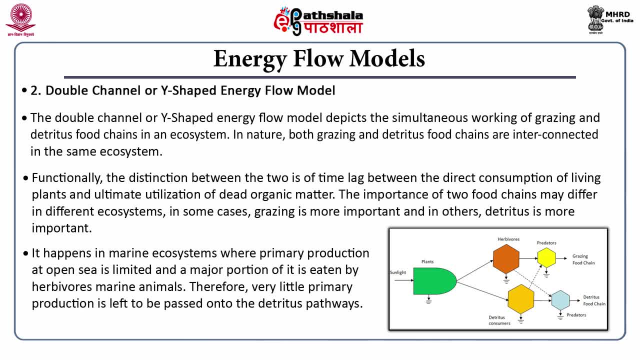 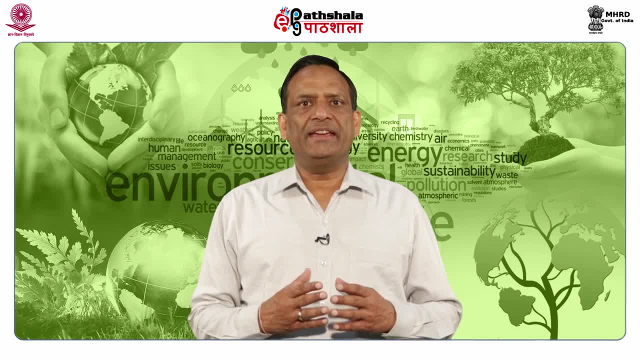 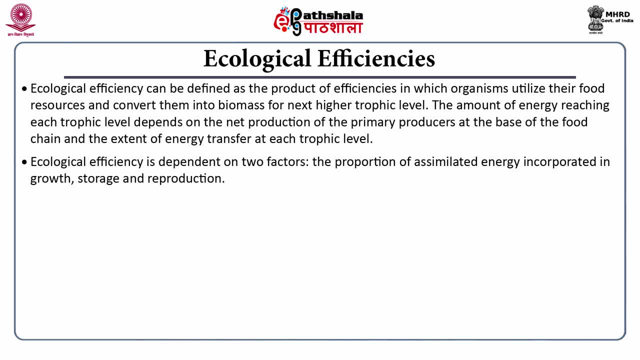 Epiodome presented a generalized model of Y-shaped or double channel energy flow that is applicable to both terrestrial and aquatic ecosystems. Ecological efficiency is dependent on two factors. Marsma Deven Accepted kalau sekot. ekologikal efficiency jest dependent on two factors. Ekologikal efficiency jest dependent on two factors. One is the production of assimilated energy incorporated in growth, storage and reproduction. The first percussion is called as assimilation efficiency, and second is not production efficiency, The product of the assimilation efficiency and the not production efficiencies, each called as gross production efficiency with an equal efficient supply. Not processing efficiency over a sonar as a result of corruption in the production. Not manufacturing efficiency over multiple facilities across the ground. NotVI Pen老ci. 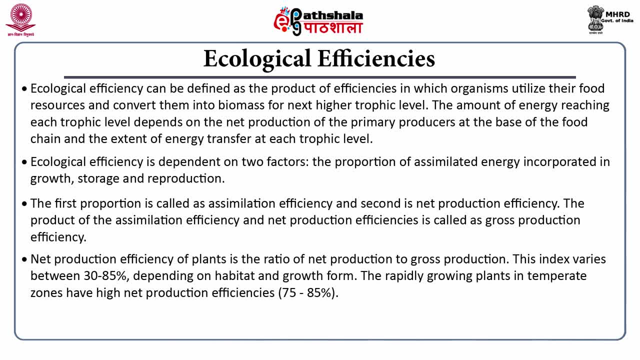 efficiency. net production efficiency of plants is the ratio of net production to gross production. this index varies between 30 to 85 percent depending on habitat and growth for the rapid grow. growing plants in temperate zones have higher net production efficiencies, in the range of 75 to 85 percent. similar 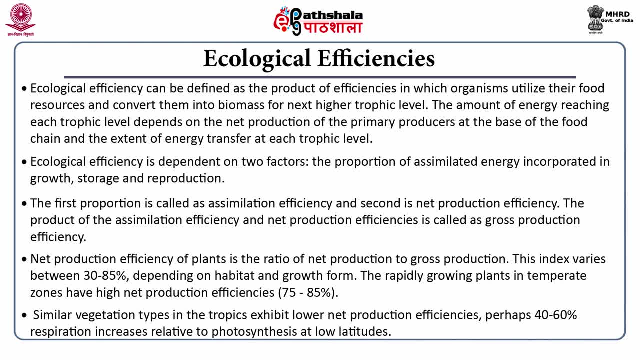 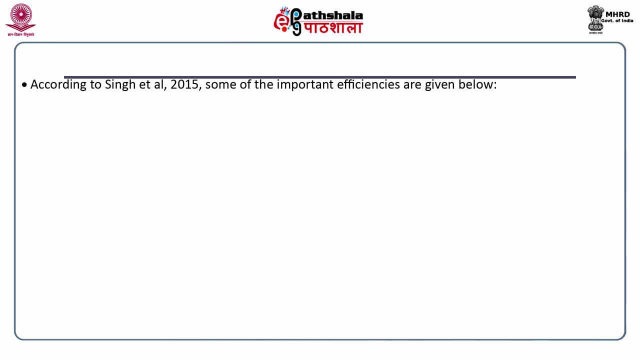 vegetation type in the tropics exhibit lower net production efficiencies, perhaps 40 to 60 percent respiration increases relative to photosynthesis at low latitude. according to Singh et al 2015, some of the important efficiencies are assimilation efficiency. this is a measure of efficiency with which a 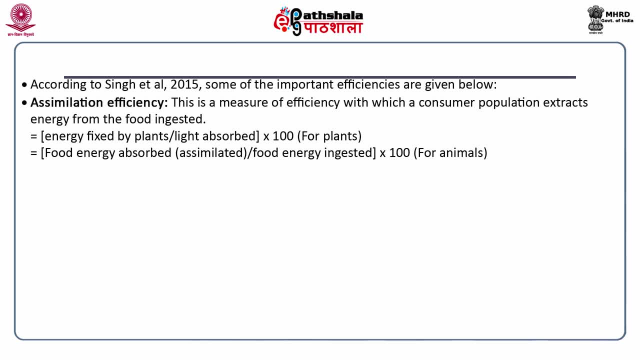 consumer population extracts energy from the food ingested. this is equal to energy fixed by plants divided by light absorbed. multiplied by a hundred is equal to food energy absorbed that is assimilated, divided by food energy ingested multiplied by hundred for animals Utilization or consumption efficiency. this is the proportion of total productivity. 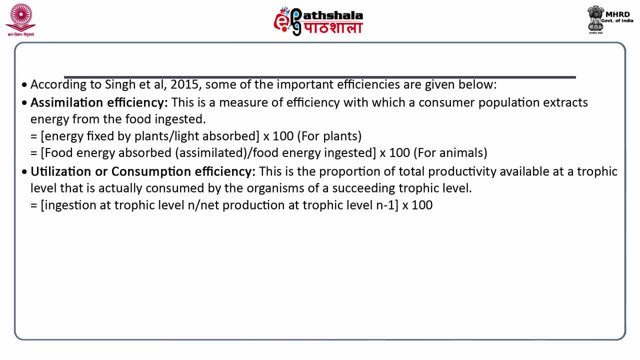 available to a trophic level that is actually consumed by the organisms of a succeeding trophic level. This is equal to ingestion at trophic level divided by net production at trophic level multiplied by 100.. Next is growth or production efficiency. This 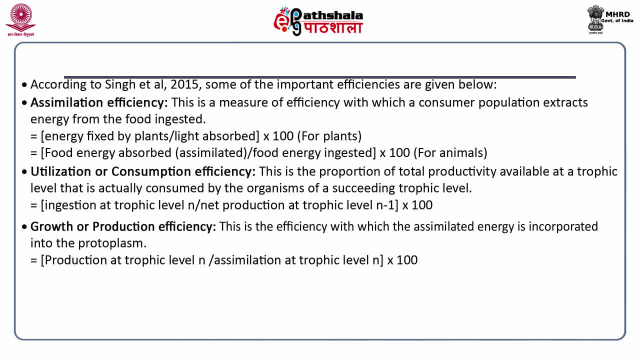 is the efficiency with which the assimilated energy is incorporated into the protoplasm. that is equal to production at trophic level and divided by assimilation at trophic level and multiplied by 100. Then we have ecological growth efficiency, and this is equal to production at trophic level multiplied by 100. 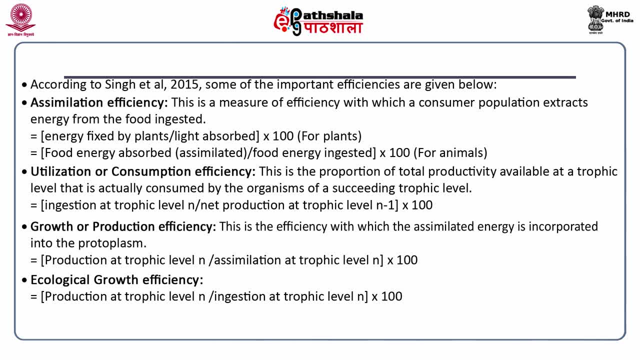 This is equal to production at trophic level and divided by ingestion at trophic level and multiplied by 100.. Then we have transfer efficiency. transfer efficiency is equal to production at trophic level and divided by production at trophic level and minus 1.. 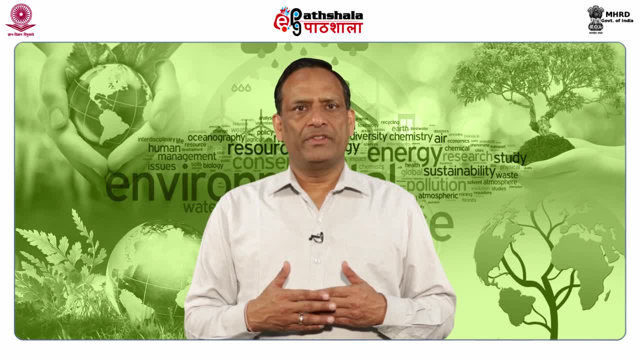 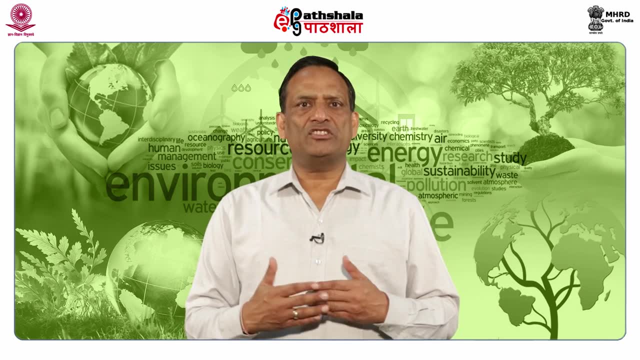 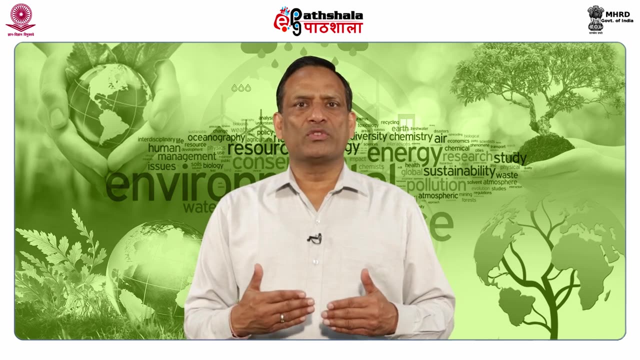 To summarize this module, the ultimate source of energy for all ecological systems is sun. The solar energy is created by heat transfer. Solar energy is captured by green plants and transformed into chemical energy and bound in glucose as primary, as potential energy, during the process of photosynthesis. 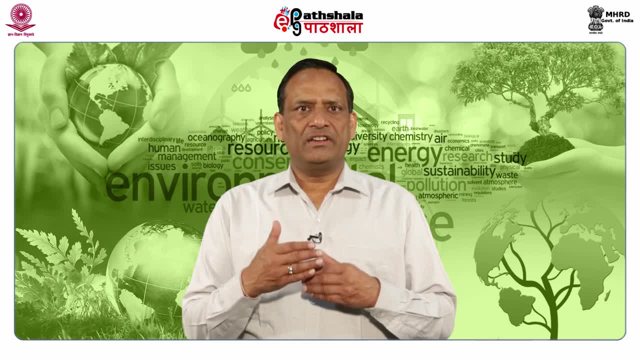 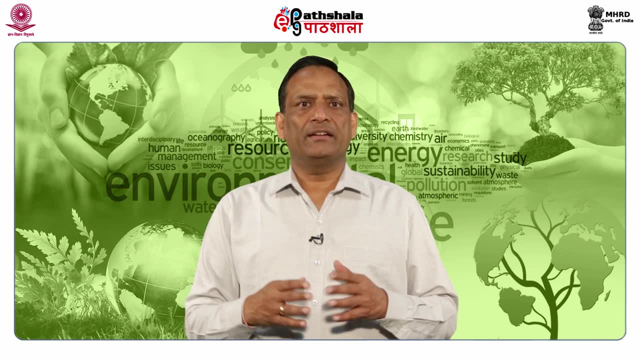 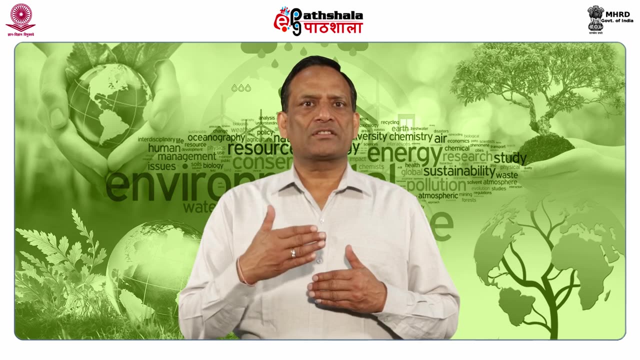 In this stored form, other organisms take the energy and pass it on further to other organisms. The flow of energy in ecosystem follows first and second laws of thermodynamics. The solar energy is captured and converted by green plants into chemical energy, confirming first law of thermodynamics. 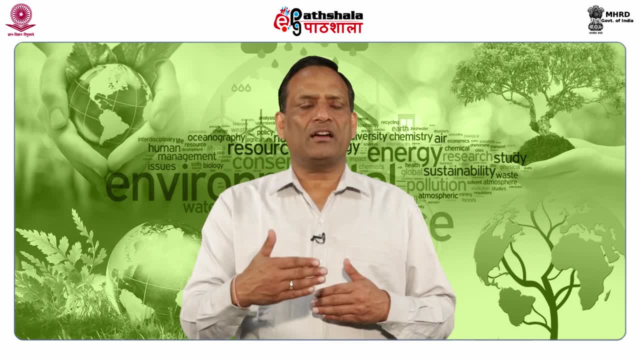 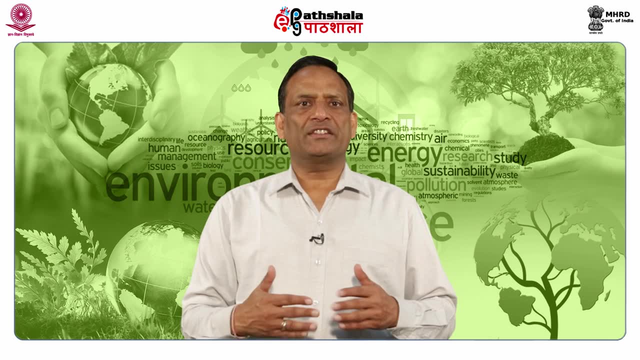 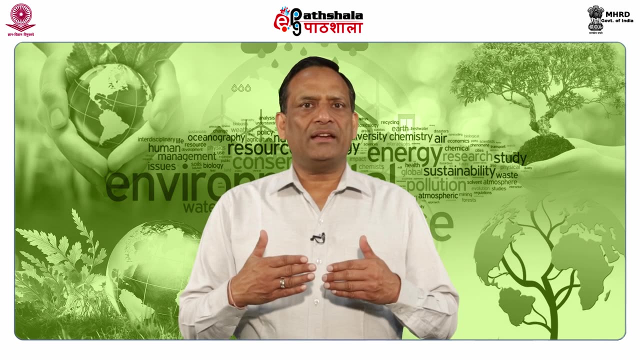 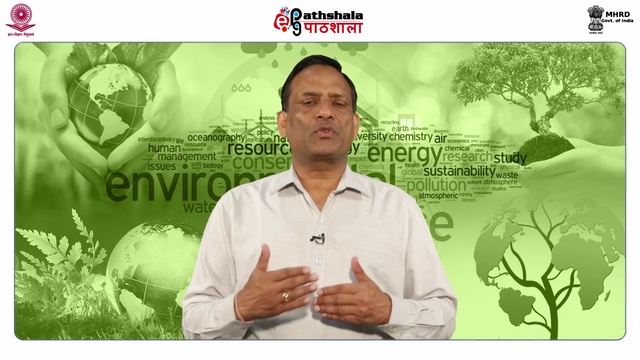 As the energy flows through the food chain, there occurs dissipation of energy. at every trophic level This loss of energy takes place through respiration, loss of energy in locomotion, running, hunting and other activities. At every level there is about 90 percent loss of energy and the energy transferred from 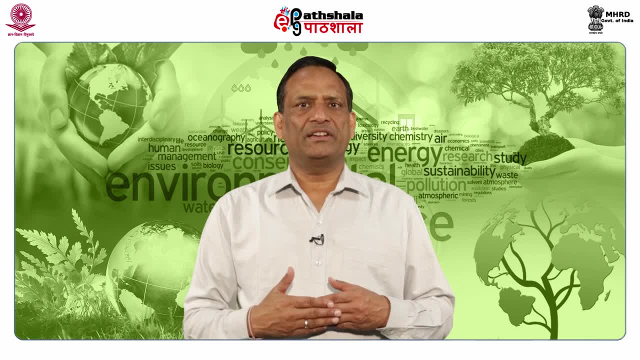 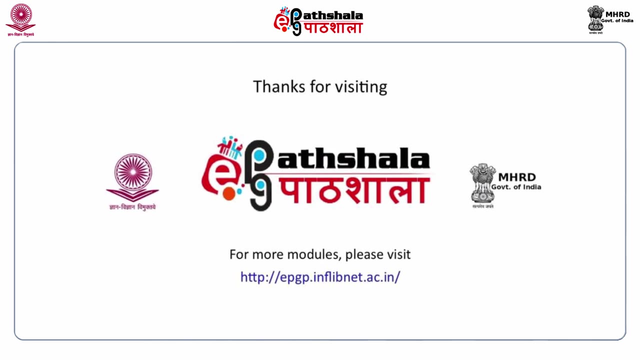 one trophic level to other is only about 10 percent. This energy flow models link the trophic levels with each other, showing the inputs and losses of energy at each trophic level. Thank you. Subtitles by the Amaraorg community.